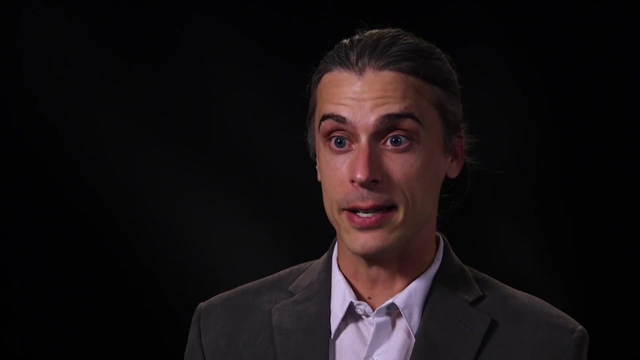 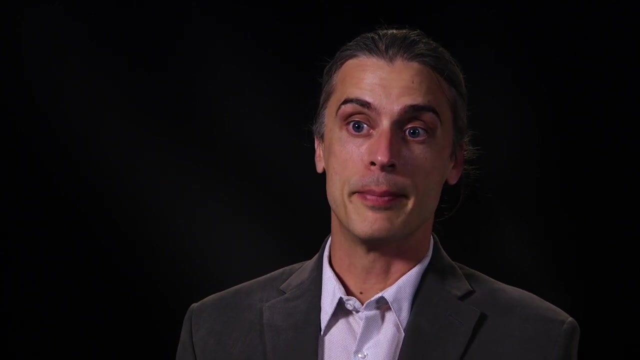 effective. One of the questions we have is: well, what's the mechanism that's driving these results for teachers that are getting low observation ratings? The short answer is: we don't really know. but there, because we don't observe it, We don't actually see what's going on between the teacher and the principal. 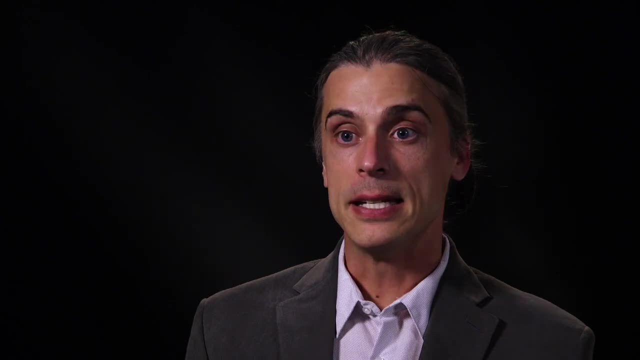 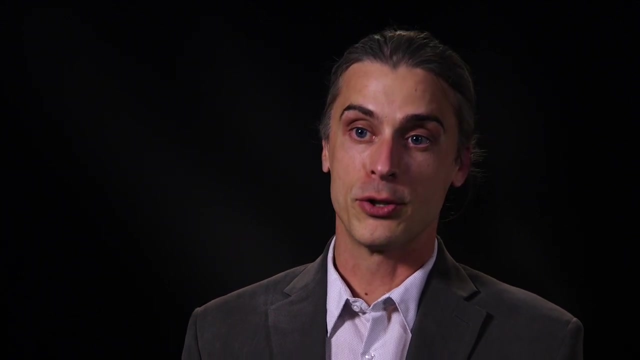 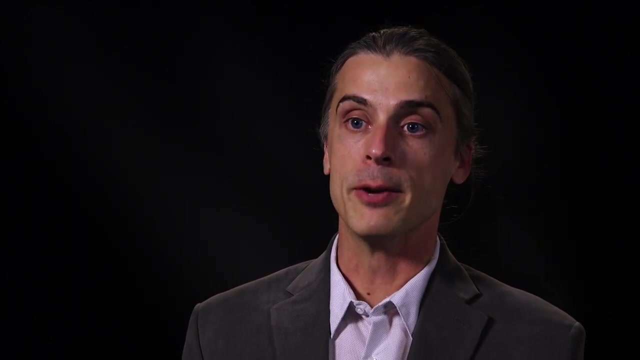 and how that retention decision is made. But there are some hints in the data. So the students that get high overall evaluation ratings but who still got very low observation scores still show this pattern. So if you got a high evaluation rating overall, you wouldn't necessarily be subject to to an 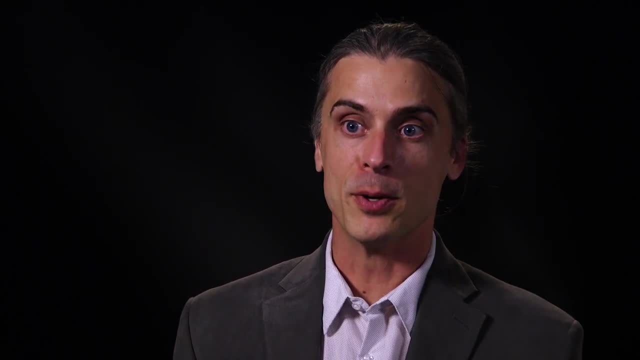 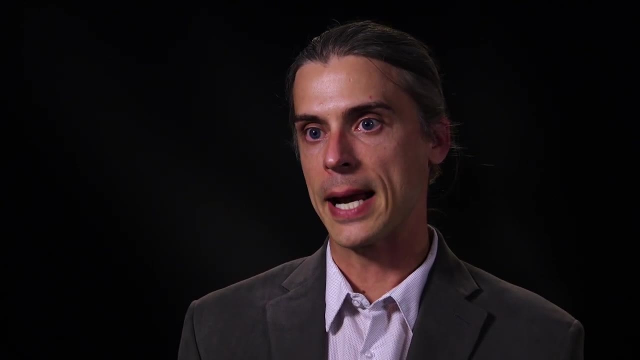 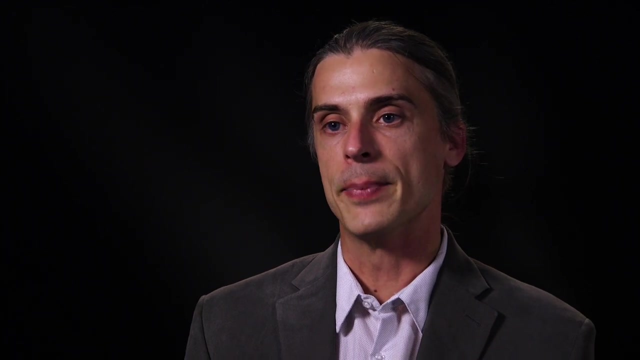 administrative removal procedure. School districts have invested really heavily in multiple measures based systems of teacher evaluation where they're collecting lots of different measures of whether teachers are performing at a high or low level, And one of the criticisms that's been raised about our systems is: well, they don't really matter because they don't. 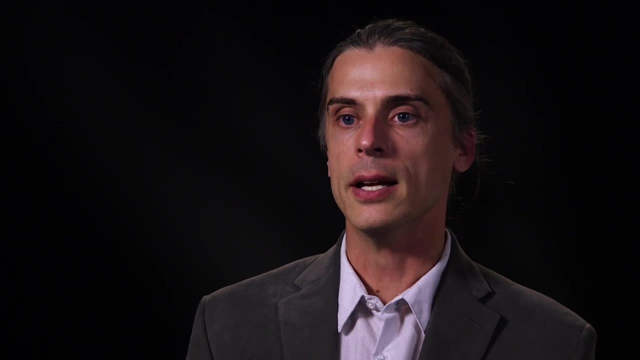 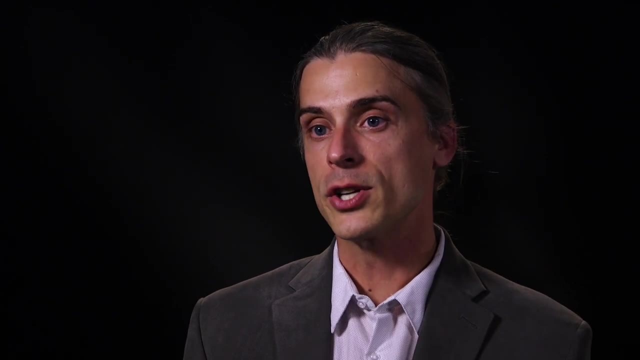 in. they don't impact teacher employment at all. We never see that anybody gets let go for low performance in in most of the states that have adopted these systems, And our results suggest that that conclusion misses a little bit of what's going on. That in fact, in schools at least, where the leadership is a very 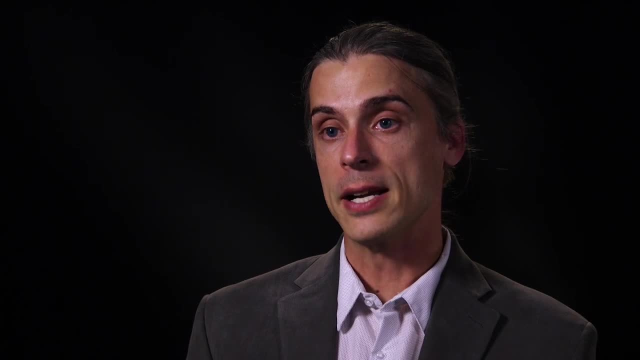 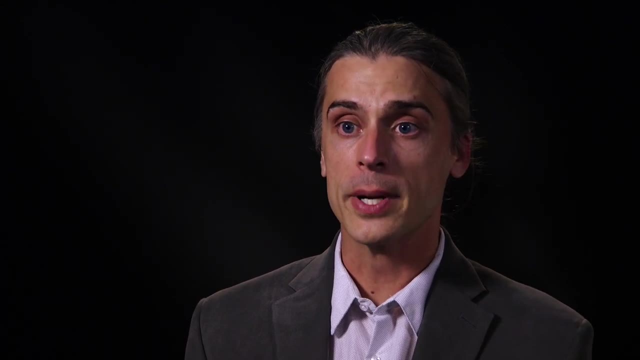 high quality. low performing teachers, as measured by their observation ratings, are more likely to leave. It's just they're not. they're not showing up on for low performance because in fact they're being counseled out. They're being moved out of that school in other ways. 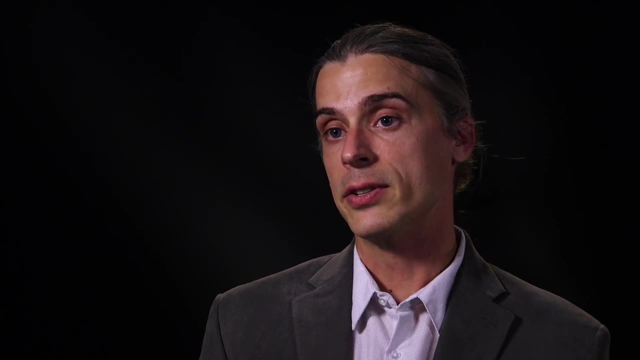 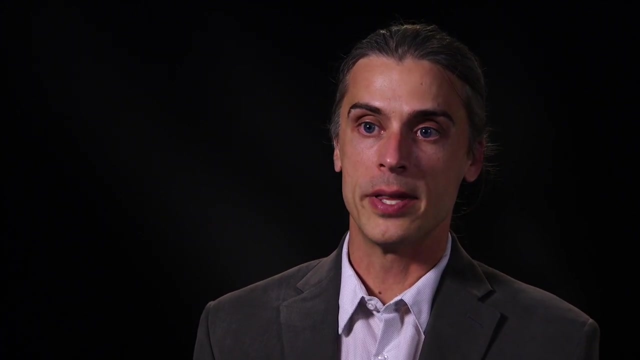 And a really interesting thing that we found is when we looked at where those teachers who left schools with high-performing principals, when we looked at where they went subsequently, what we found is they didn't just show up at other schools within the same school district. 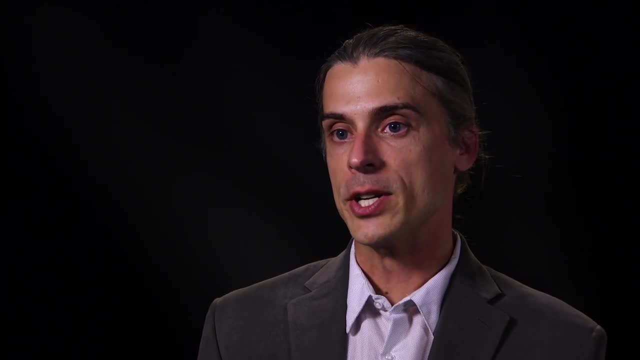 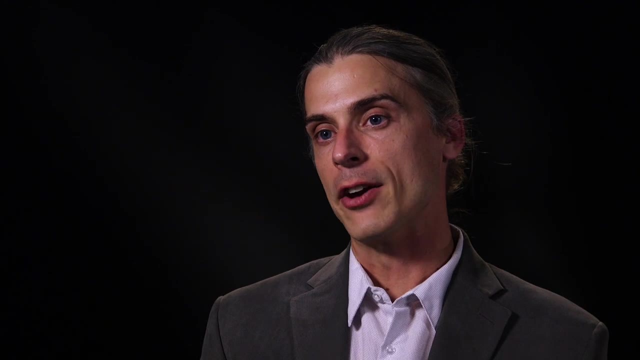 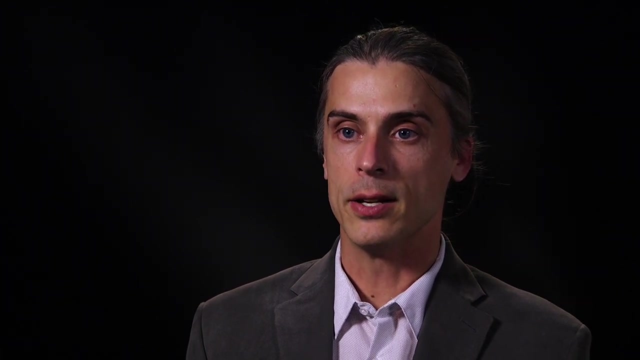 They usually exited the system which suggests that high-performing principals are. you know, when they have a low-performing teacher in their school, they really are getting them out of the educational system altogether. This relationship that more effective principals tend to be associated with higher turnover- 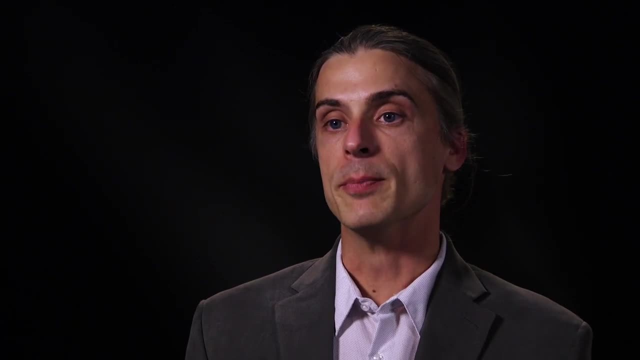 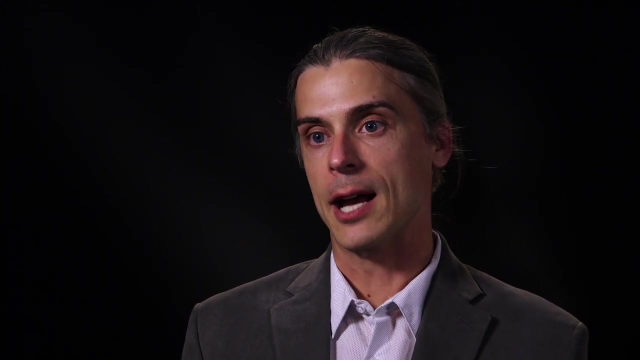 rates among lower-performing teachers really is most evident when you look at performance as measured by observation scores. The reason that's important is because principals are the ones that are collecting observation scores, So what we interpret that as showing is that effective principals going to classrooms.